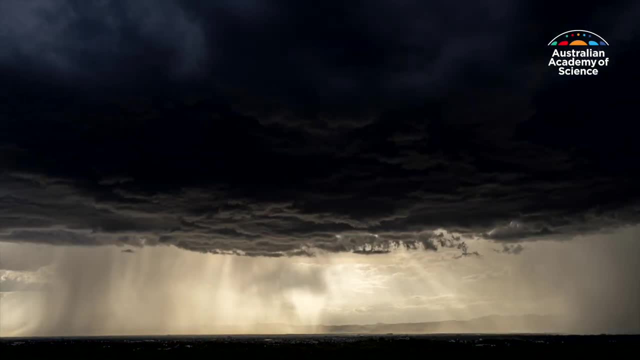 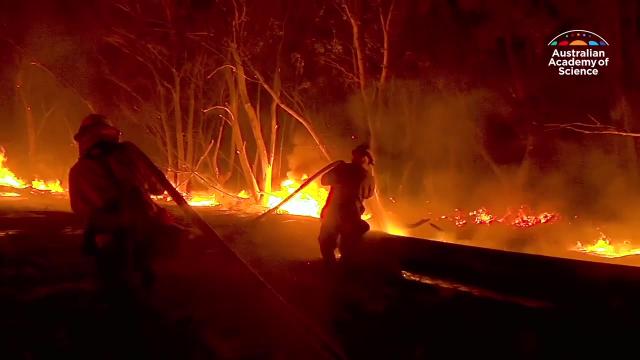 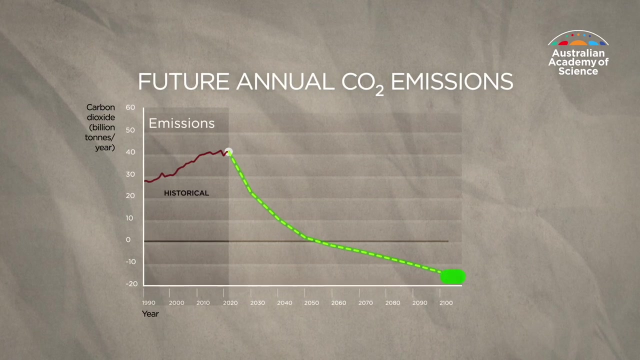 The impacts of climate change are being felt around the world, From extreme weather events to biodiversity loss. we've been put on notice to take urgent action. Countries including Australia have committed to limiting global warming to well below two degrees above pre-industrial. 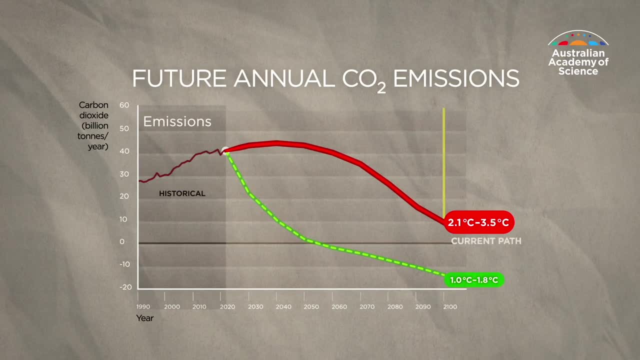 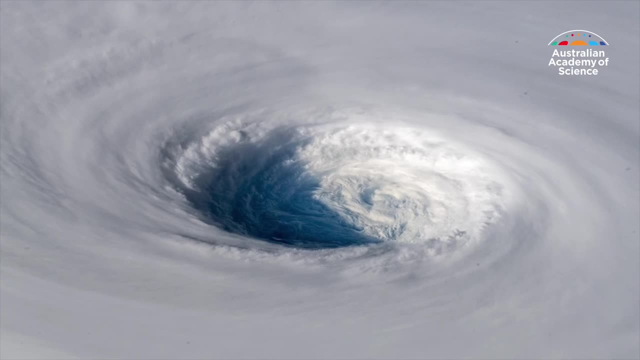 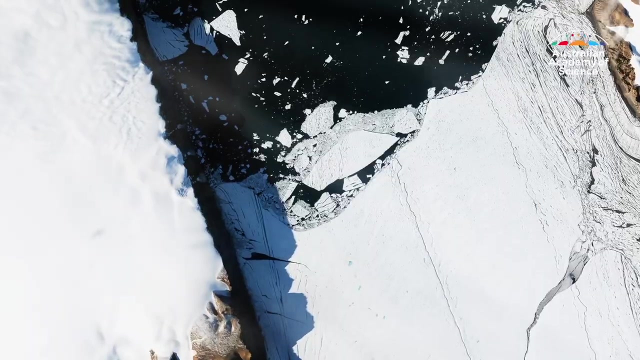 temperatures, But right now we're on track for 2.1 to 3.5 degrees of warming by 2100.. That's beyond what scientists consider manageable and could have potentially catastrophic impacts for the environment, people and the economy. So what we have is a world which is increasingly 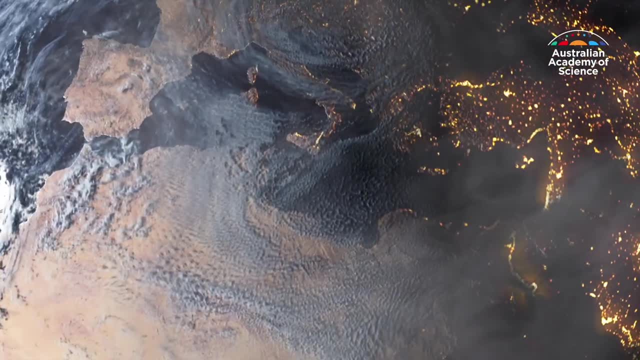 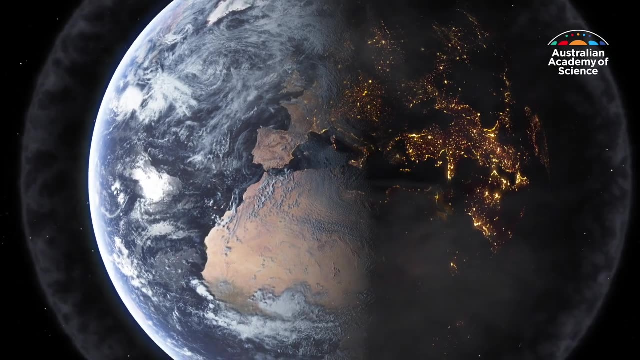 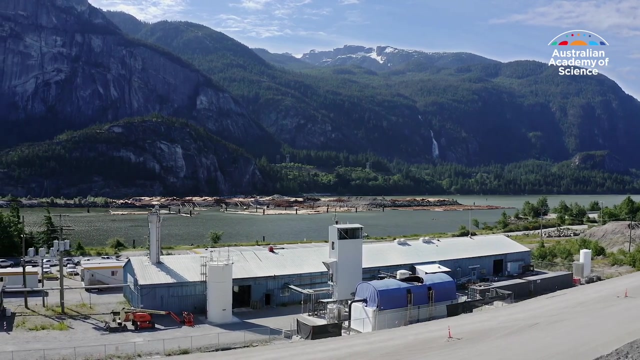 stressed by human activity. The solution is to address the tens of billions of tons of greenhouse gases being pumped into the atmosphere every year. That requires not just dramatically reducing future emissions, but removing greenhouse gases already released. This means drawing down or removing these historical emissions from the 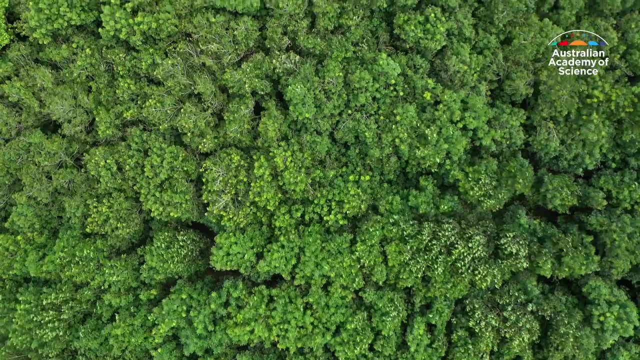 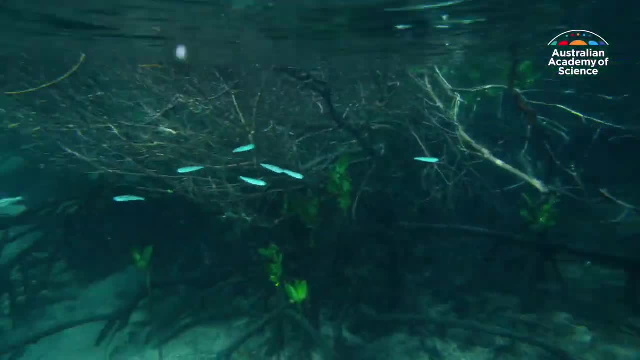 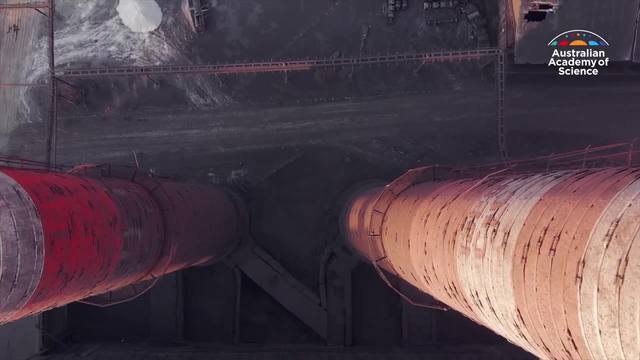 atmosphere for, if you like, geological time. Natural systems such as our oceans and forests are highly effective carbon sinks, but they need help, especially given the further pressures from events such as bushfires and ocean warming. We don't yet have the right toolkit to effectively. 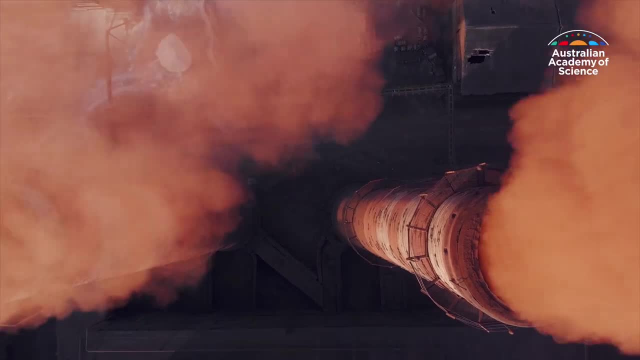 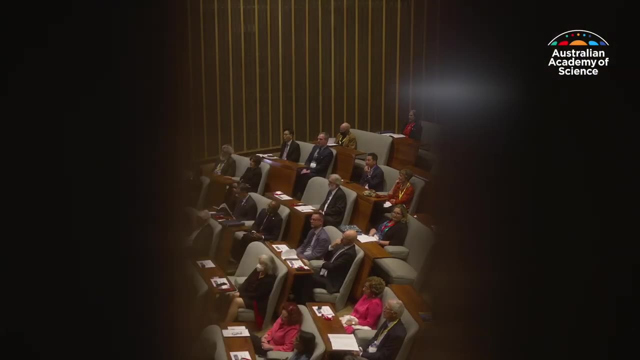 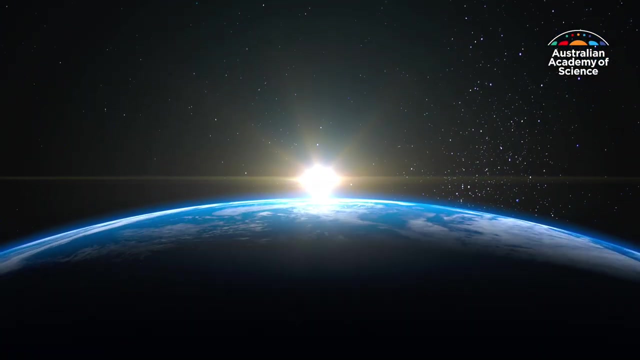 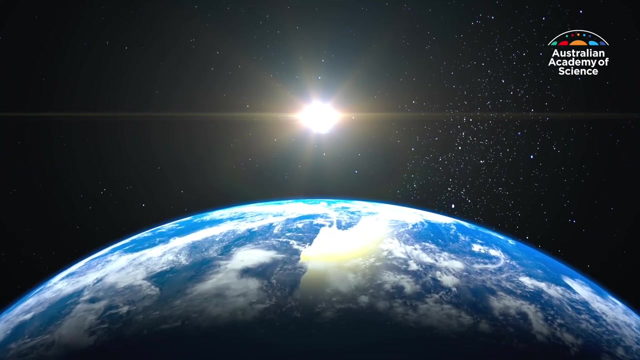 remove greenhouse gases at the scale required. So the Australian Academy of Science brought together the country's leading experts to identify opportunities to expand research efforts and start the conversation in Australia. Beyond strengthening existing carbon sinks, new technologies will need to be developed. I think the scale of the problem that we're facing means that we can't discount anything. 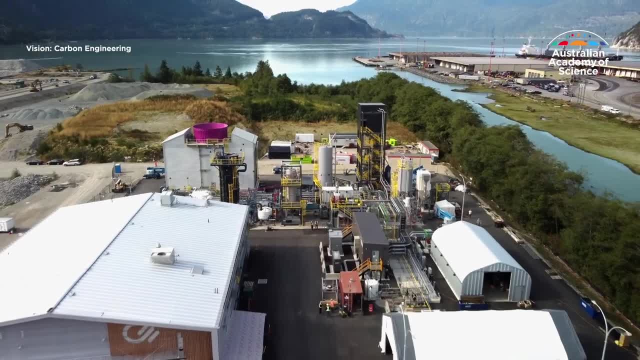 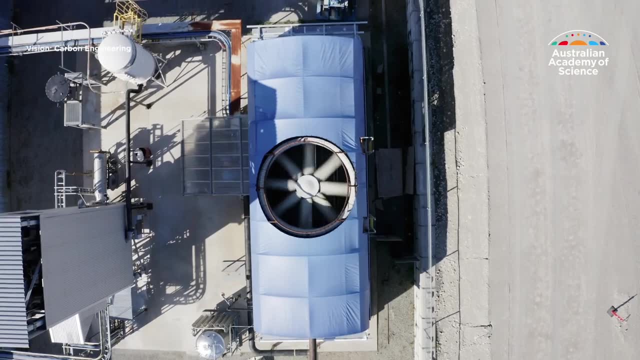 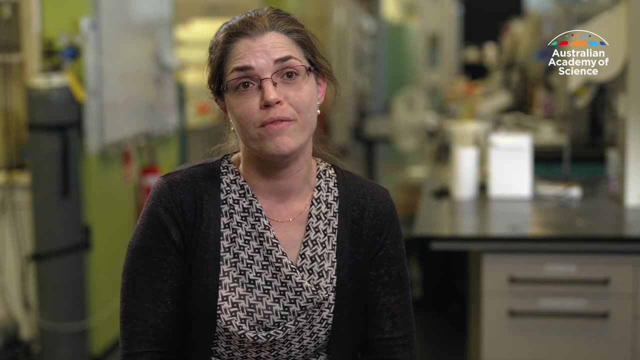 and, in fact, everything needs to be on the table, Including things such as climate change, such as direct air capture, a technology that mimics trees. We can develop these nanoporous materials that are really highly selective for capturing carbon dioxide from the atmosphere and other greenhouse gases. So, in the same way that 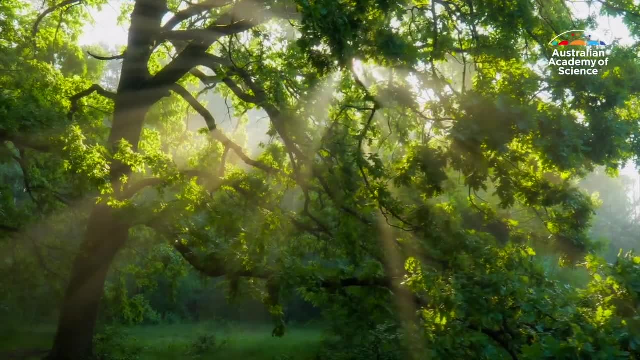 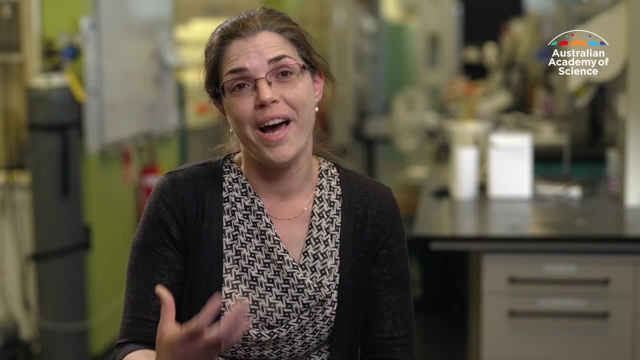 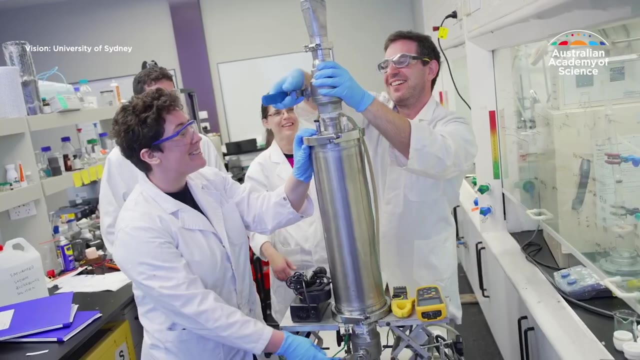 a tree uses photosynthesis. it takes in carbon dioxide and processes that carbon dioxide and spits out oxygen and energy at the other end. we've got a way to do that, if you like, using technology. The first air capture units in Australia, designed by Southern Green Gas, are now in.